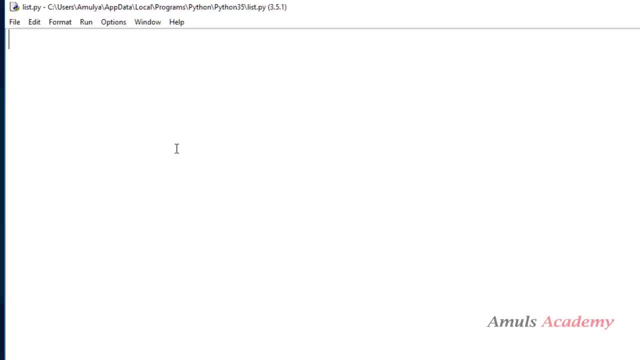 I will show you the example. so first i will take a single list. So if i want to find out the maximum value, i can just print max of list 1.. So i will save this and run this. it will print 78, the maximum value in this string. 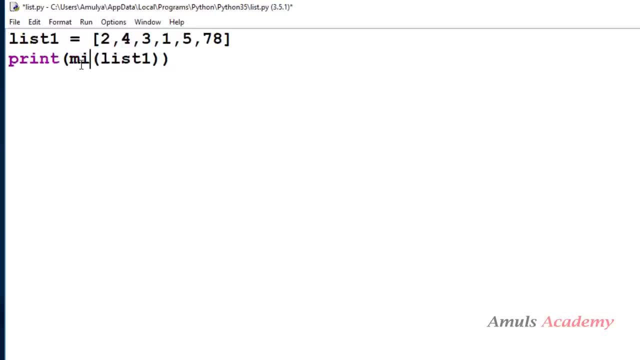 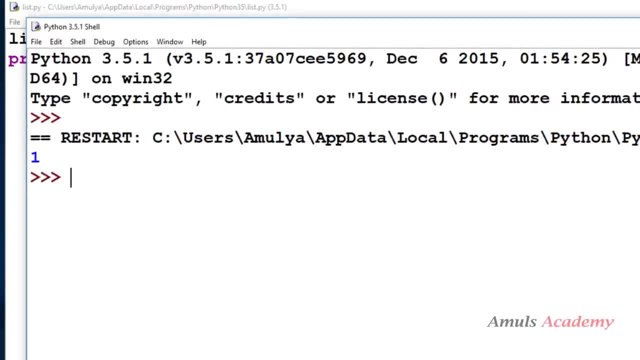 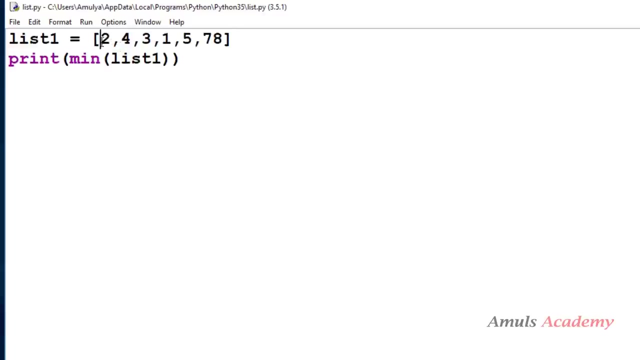 If i want minimum, i just can mention min and it will print 1.. So 1 is the minimum value in this list, one 1. is the nested list, for example? ok, so now, if i save this and run this, we will get the error. 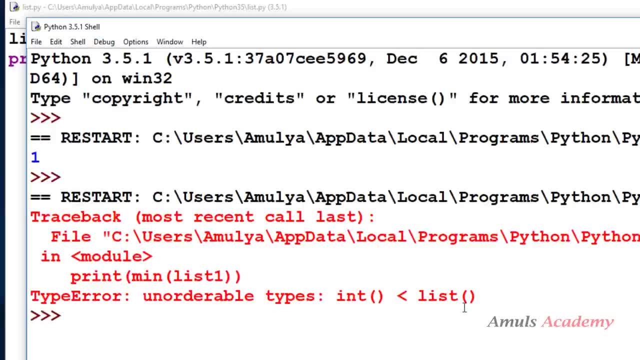 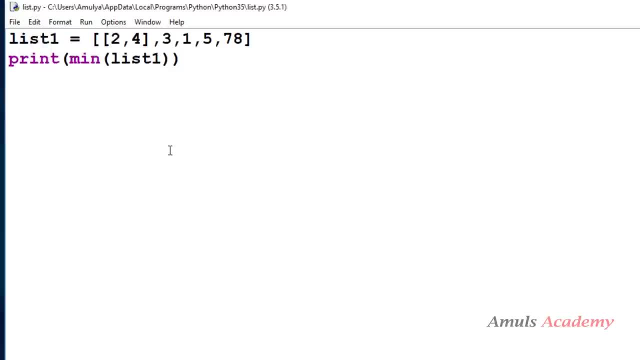 because we can't compare the integer with the list type. so then now, how to find out the maximum or minimum value in the nested list. so for this, what we can do is we can convert the nested list to flat list first or single list first. then we can use this max or min functions. 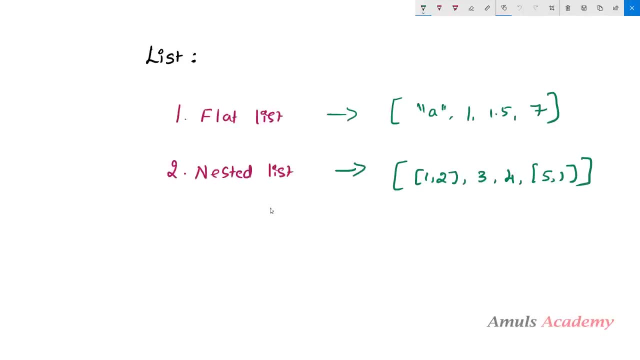 as we know, this max and min function won't work for the nested list, so what we will do is we will convert the nested list to flat list first. then we will apply that max function or min function to find out the maximum or minimum value. ok, 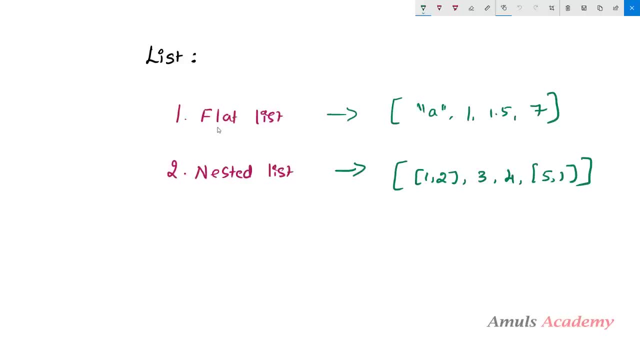 so how to convert this nested list to flat list, then, and that we will see in the program. so here, first we will define the function which will return the maximum value. so i will take the function name as getmax. it will take list to find out the maximum. 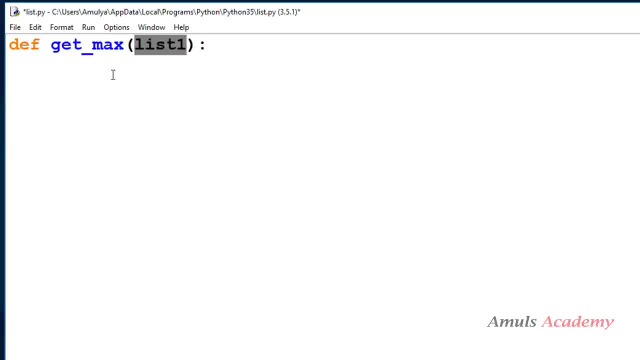 value in the list. we need list, right. that's why this parameter list1, and next here i will go through each list, each element of the list. ok, that's why this for loop. i want to go through the each element at a time, so for i in list1 that is nothing, but first i value will be the first element. 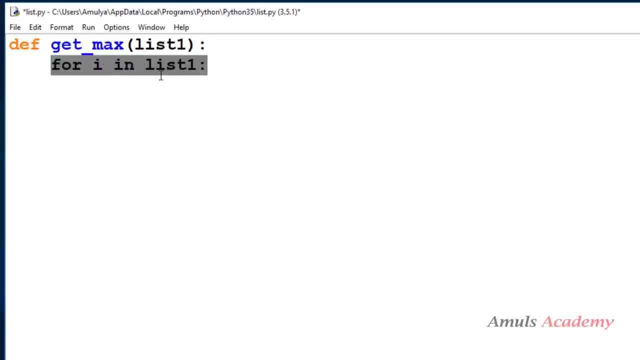 of the list1. next second element of the list1: ok, like that. and for each element i will check the type, whether it is of integer type, float type. ok, so we will check the type of the each element if the type is list, ok. so then i will again call this function. 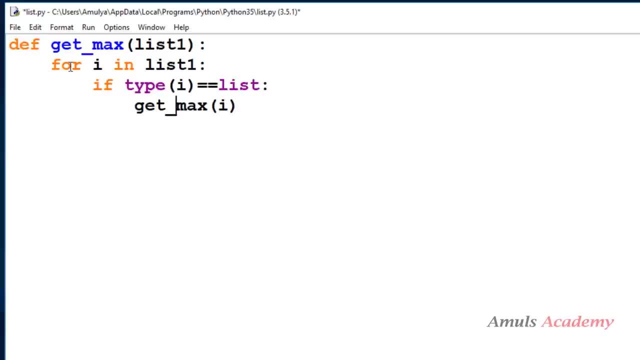 so here what we are doing is we are taking the list and we are going through the each element of the list and we are checking the type of each element. if the type of that element is list, then again call this function. that is nothing, but again go through this steps. 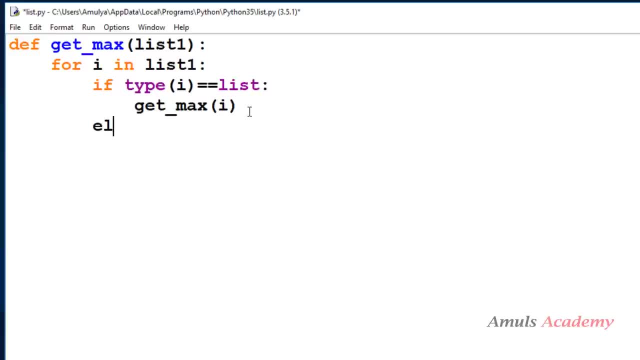 ok, if not ok, then i will take a list, ok, a new list here. initially i will take a list called list2 and it will be the empty list which will store the flat list. so this is the process of changing the nested list to flat list. 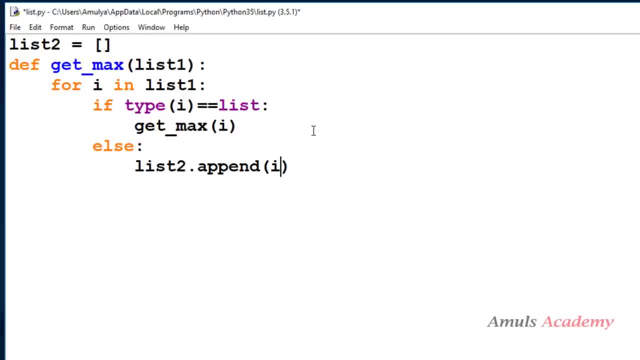 here. what i am doing is i am going through the each element of the list. if the type of that element is list, then again i am going through the each element of that list, inner list. if the type is not list, then i will append that value to a new list that is list2 then. 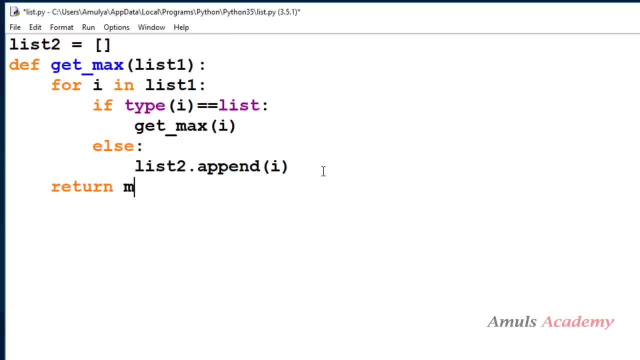 finally i will return max of list2.. ok, ok, once finally list2 contains all the elements in the flat list or in the form of single list, then we can apply this max function on that. so next here i will take the list1. i need to take the nested list. 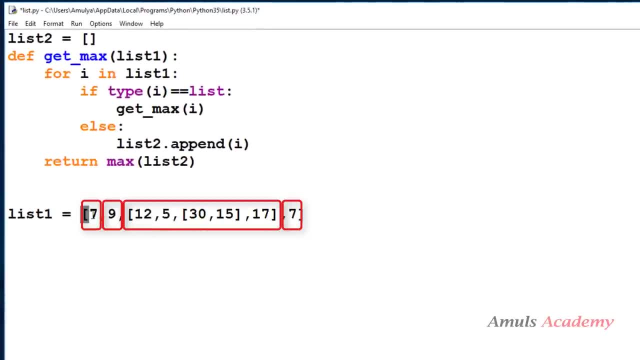 so this will be my list. ok, so this is the first element. second element: this will be the third element. third element, which contains nested list. ok, this will be the fourth element. in this nested list, we can see the first element, second element and this is the third element. 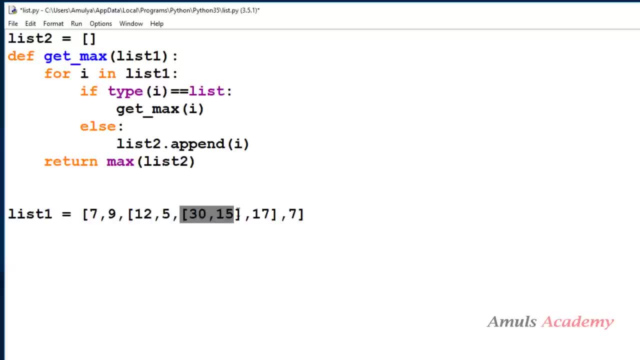 and this will be the fourth element, and this in this nested list. this will be the first element and this will be the second element. so now i will print: get max list1.. ok, ok, ok, so here. why i am printing this function call is because it will return the result. so i 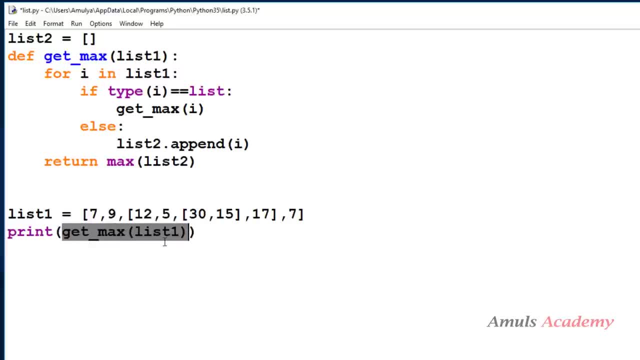 want to print that result right. that's why i am printing this function call. this is the function call, so it will go to here and it will execute this part. so now, if i save this and run this- so maximum value is 30- we will check that. 7,, 9,, 12,, 5,. 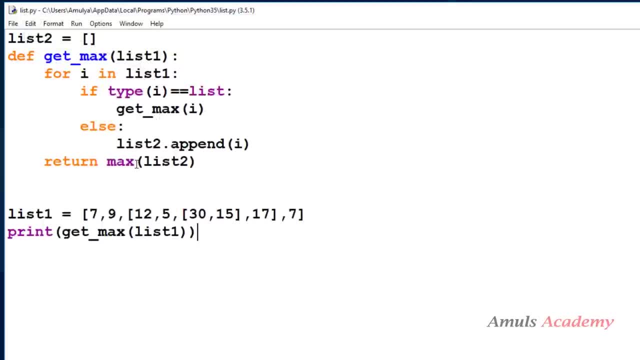 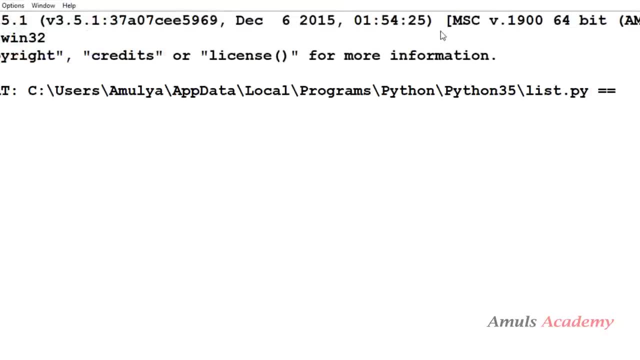 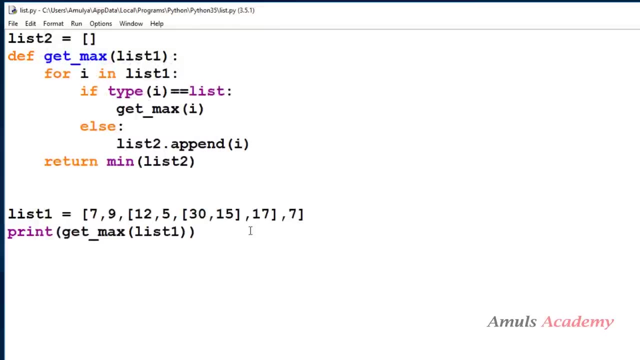 30,, 15,, 17 and 7. true, right, 30 is the maximum value. if i want minimum value, can take minimum minimum here: 5 minimum is 5, 7, 9, 12, 5, yes, true, right, so in this way we can find out the maximum. 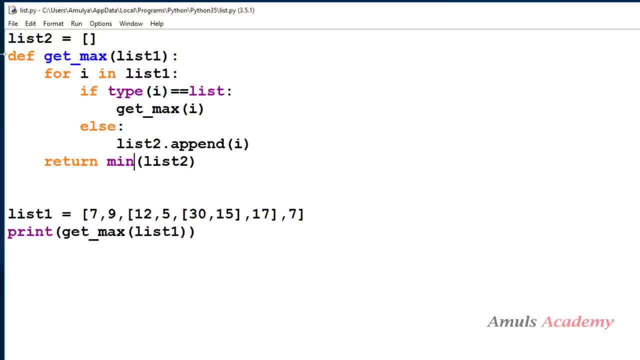 or minimum value in the nested list. so here, what will happen is: first, this will be executed: list2 is an empty list. next, it won't execute this function definition. this function definition will execute only when it is called ok. so now it won't execute this. it will execute. 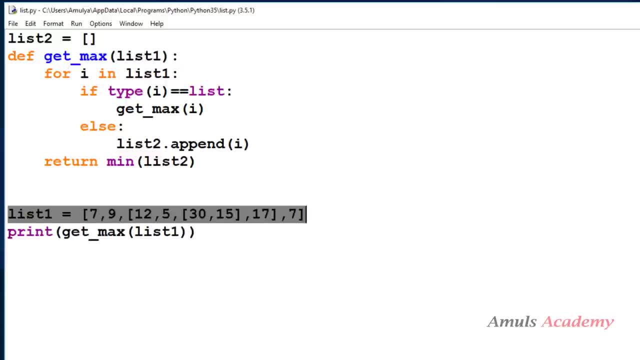 this. ok, list1 is this. next here we can see print getmax list1. getmax is an function call, so control will go to here. ok, to this function definition. so here list1 is this. so here for i in list1. so i is 7 first. so it will check whether type of i is list, whether type of 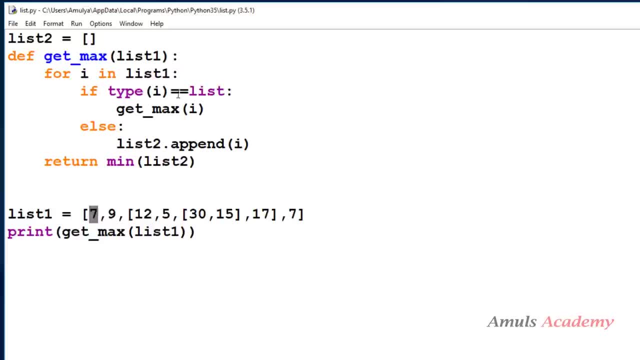 7 is list. no 7 is int. it is not list, so its type is not list. so it will execute else part and it will append this 7 to new list, that is list2. ok, so list2 contains 7. now again this for loop will work. and now 9. i value is 9, so it will check whether type of 9 is.